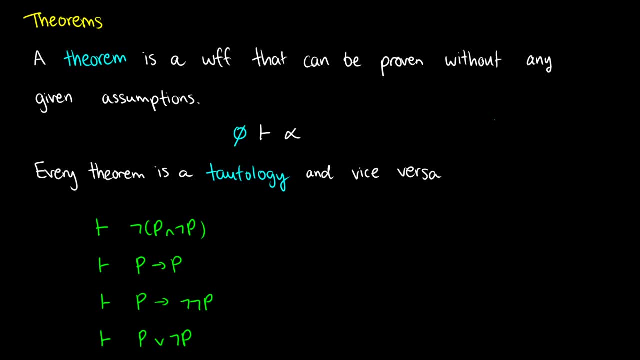 So we need to essentially start with no assumptions whatsoever and then create a proof. So we're going to do that for these four in this video. So the first one: I want to show that p arrow p is a theorem, So I can still use all the rules as before. I can use 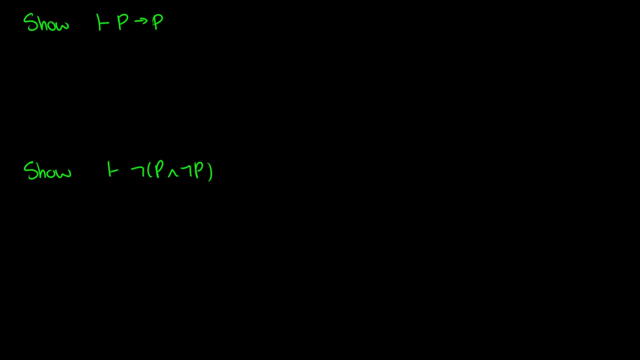 c p, r a, a. I can use and introduction and elimination and all those things. So instead of having an assumption that we start out with we don't have anything. So what I can do to start is: I can still make assumptions. I can still make assumptions for c p. 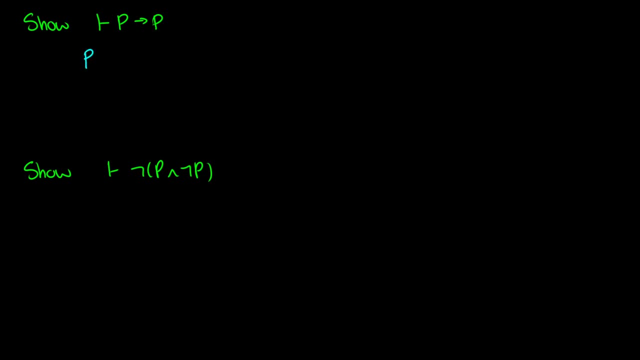 and for r, a, a, that's fine. So what I'll do is I'll start with an assumption, a hypothesis for c, p, So this just isn't given anymore. It's not information we start with that is guaranteed to be true, It's just a hypothesis. So we can set this up now. Okay, well, if we have p, 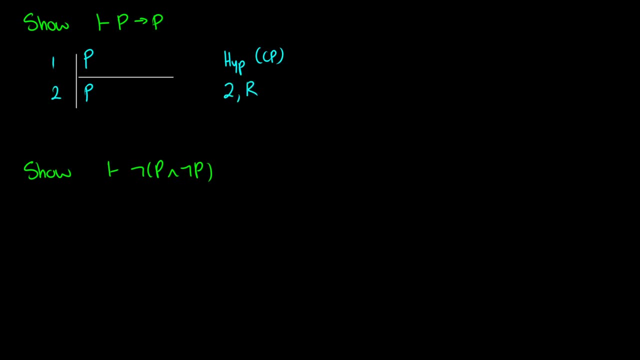 then in line two we can just reiterate it. So two is a reiteration. And then in line three, p arrow p out, because from one to two, through a conditional proof we got that if we assume p then we get p. So this would be the proof that p arrow p is a theorem. So notice how there's no line. 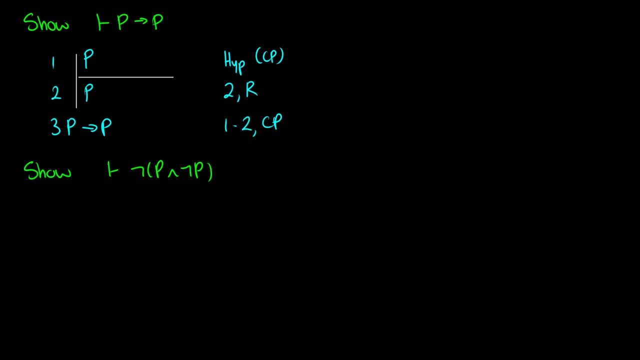 to the left of this, And that's because when we introduce that line in our other proofs, usually we have some assumptions And then we end up with something at the end. So this is our consequent. But when we have the line to the left of this, we get the proof And then we get the 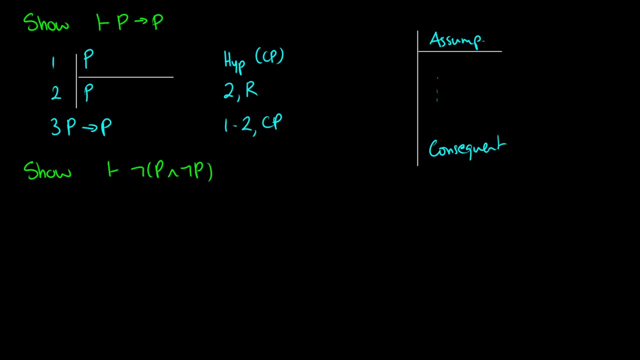 left. That means that we have assumptions, that we used to get that consequent. But in this case, on the left here we only have our line when we introduce our subproof, When we go out of it, we don't have any assumptions to begin with. So p arrow p is just on its own. It's the theorem. 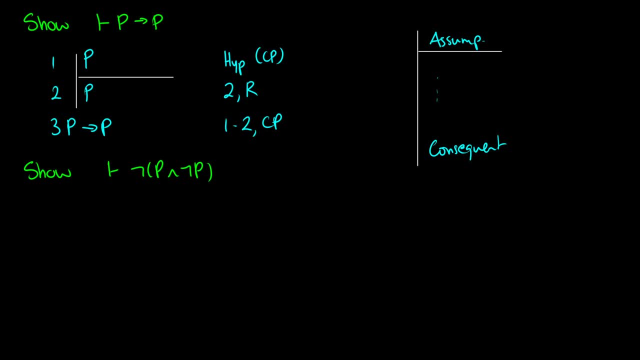 Okay, let's try. not p and not p. Let's prove that. Well, we can still use strategies here. So if I need to get not p and not p, I'm just going to assume p and not p and hope that we can negate. 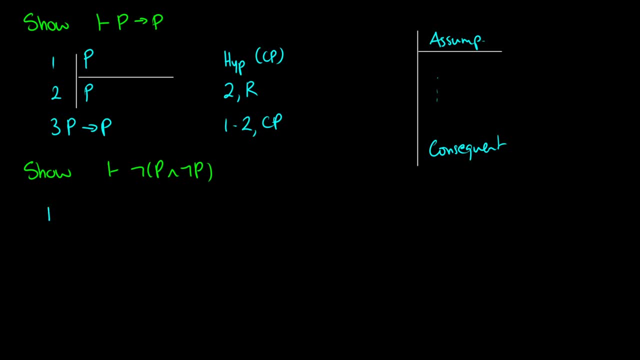 it with a contradiction. So that's what I'll do. In line one I'll assume p and not p. So this is a hypothesis for contradiction. I want to prove that this is going to give us a contradiction, So we can negate it. So we'll start an assumption here. 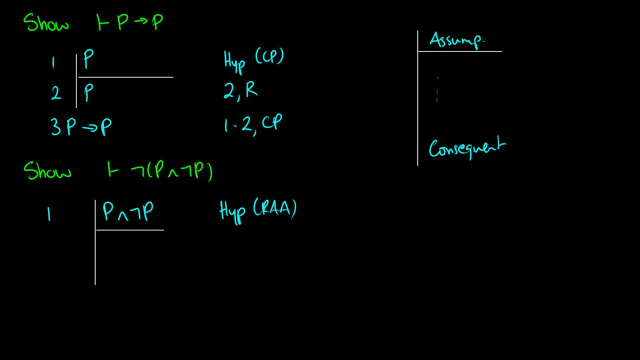 Okay, well, if I have p and not p, that gives me a contradiction by definition. So actually I can redraw this a little bit. If I have p and not p, then in line two I can negate this and I can get p and not p And from one to one. that was a proof by contradiction. 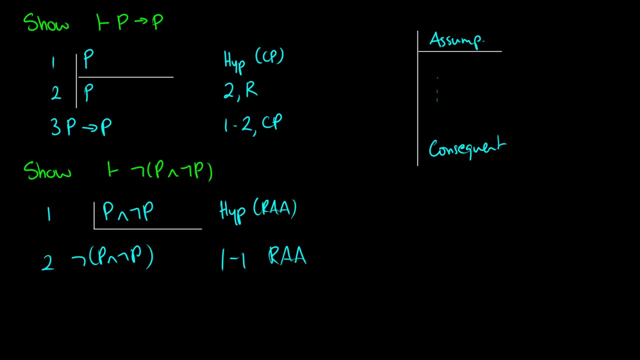 because p and not p itself is a contradiction. I guess, if I want to make this a little bit more explicit, what I could do is in line two and line three I could use and elimination on one to get p not p, And then in line four I can then claim that this is a proof by contradiction. 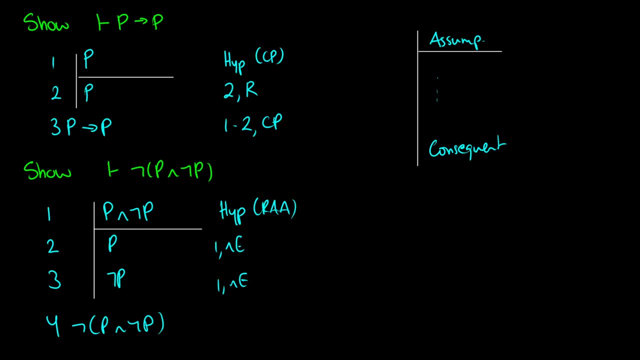 because I have p and I have not p. Therefore the assumption must be false. So from one to three, that is RAA. That'd be another way of doing it where everything is explicit. But again, we started with no assumptions. We did a subproof where we assumed RAA, p. 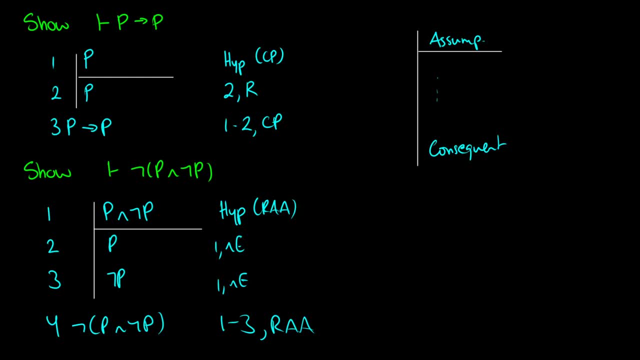 and not p for RAA. and then we found it, But we didn't need any initial assumptions to get to not p and not p. We didn't need any initial assumptions that were given to us for free to get p arrow p. This isn't dependent on whatever we're given. Okay, let's do the proof. 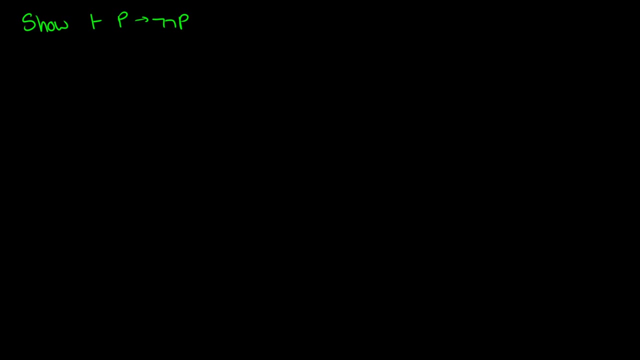 that we have p arrow, not not p. So what I will need to do is I will need to assume p for a CP proof. It's a conditional proof. I have p arrow something, so I need to assume p. Okay, who knows how long this will go. Let's say it's very. 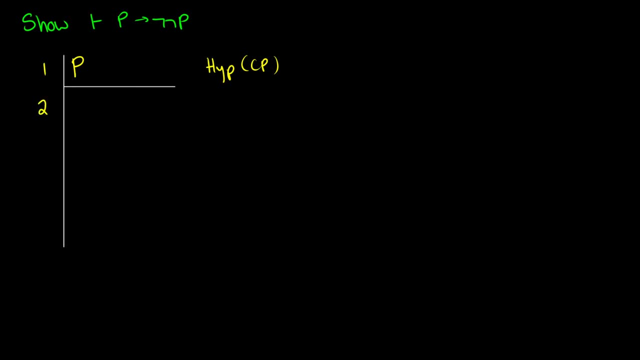 very short here. Two: what am I going to do? I need to get not, not p. So what I'm going to do at this point is I'm going to assume not p for RAA. I want to get a contradiction here with not p, And I think I'm going to have a fairly easy time getting this. So in 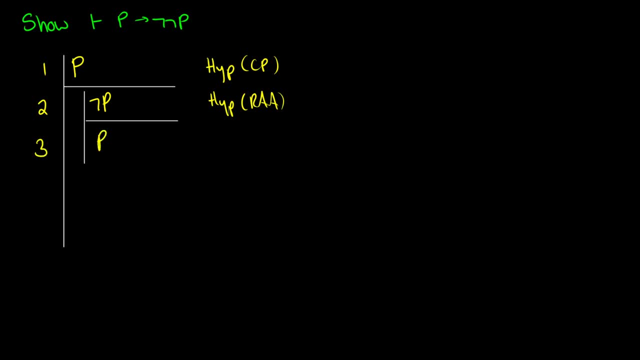 line three, I'm going to reiterate p from one, So that's one reiteration. Now I have p and I have not p, so I get a contradiction, Or I can get not, not p, And this comes from two to three by RAA, because we assume not. 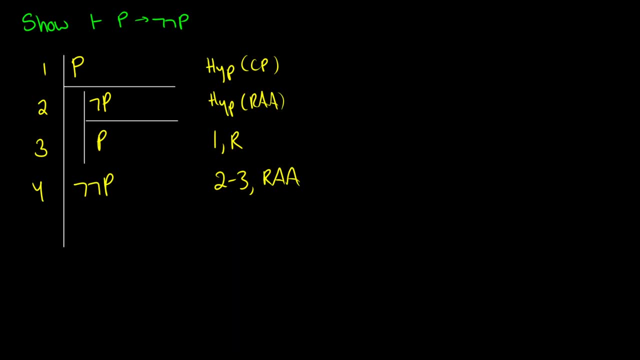 p and we get p, And now we have p to not not p from one to four. So on line five I can write: okay, if we assume p, we show that we get not, not p. So this is one to four. 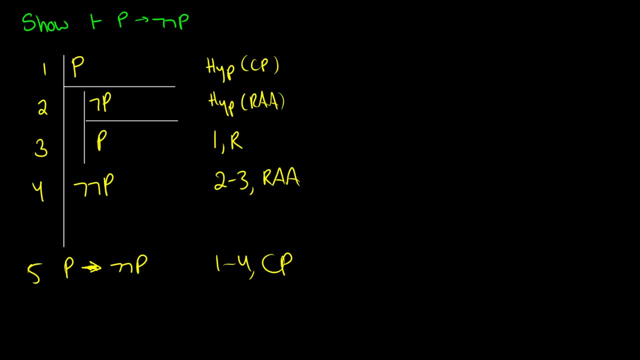 And this is a conditional proof. This means whenever we want, we can introduce p arrow, not not p. This is like doing double negation in the opposite direction. Imagine that I'm somewhere in a proof, So let's say I'm doing a proof And I have q or p And I'm trying. 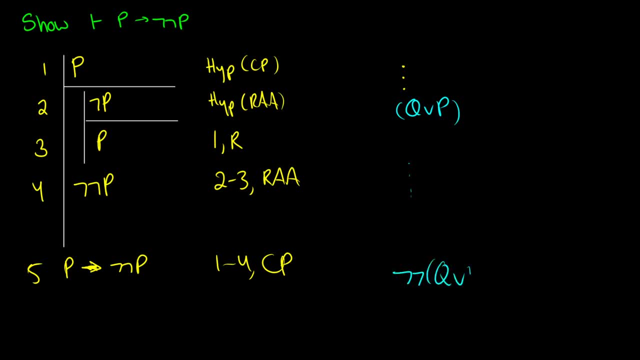 to get at some point. not not q or p. Well, double negation just takes away the two negations. But what I can do now is I can introduce, say, a theorem somewhere in line j that says: okay, if I have q or p, then I have not, not q or p. 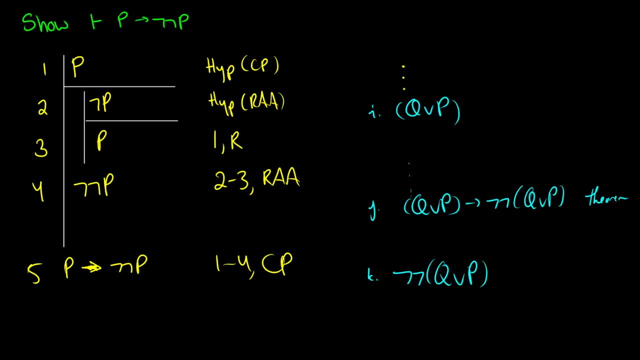 This is just a theorem. It's a theorem from what we showed now. So then in line k I can use that theorem on q or p to get not, not q or p. It speeds things up. Okay, One more that we'll do. We want to show that p or not, p is a theorem. So we want to show. 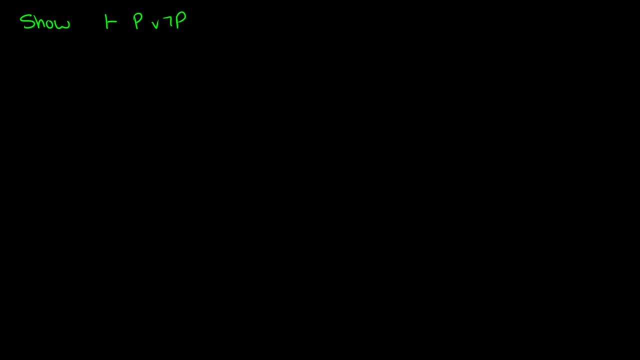 this is true. So what I'm going to do is I'm going to assume the negation for contradiction. assume that not p or not p is true. This is a hypothesis that we will use for a contradiction, So that'll be line one, which means we have to introduce our line here and our assumption. 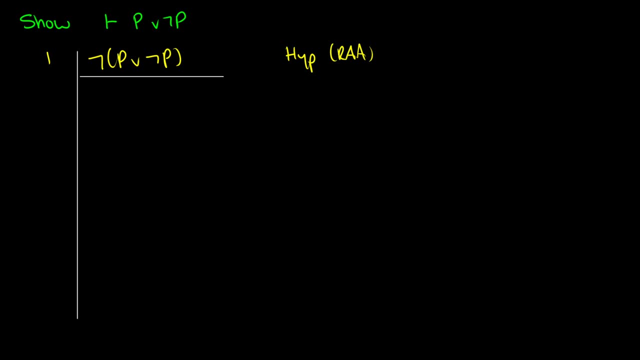 Okay, now we need to get p or not p at some point. So I think I'm going to use not p or not p as a tool for contradiction. So what I'm going to try to do is I'm going to try to get p or not p. 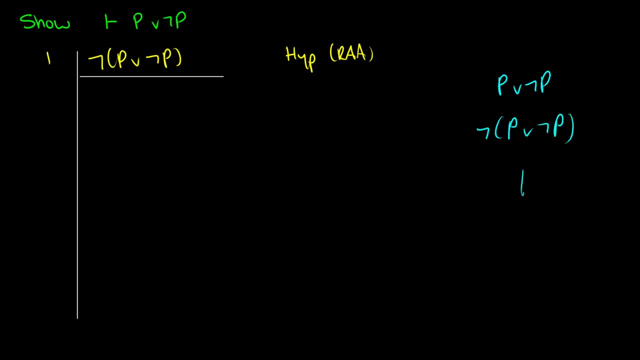 along with not p or not p, So I can get a contradiction and negate some things. So that's my goal, Okay. so I think what I'll do is I'm going to assume p for ra. Okay, well, I'll just assume p. 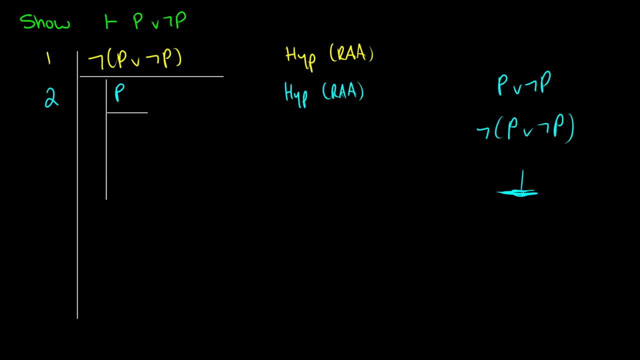 So I should set this up. They only need three lines. So in line three I'm going to use or introductory To get p or not p. So from line two, or introduction to get p or not p, And then for I'm going to 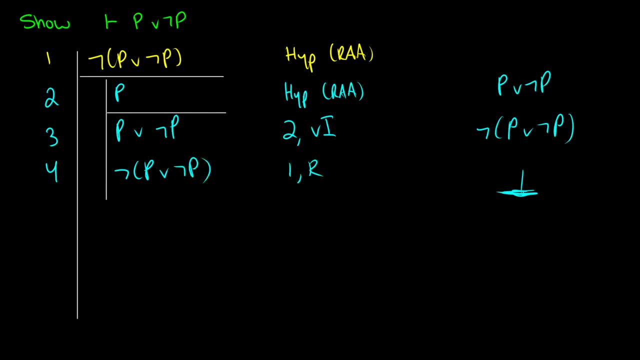 reiterate the assumption. So from one I've reiterated not p or not p. we have a contradiction now. So then, in line five, I can claim not p, And this is from two through four, And this is a ra proof. Okay, so I've not p. Well, this is good. 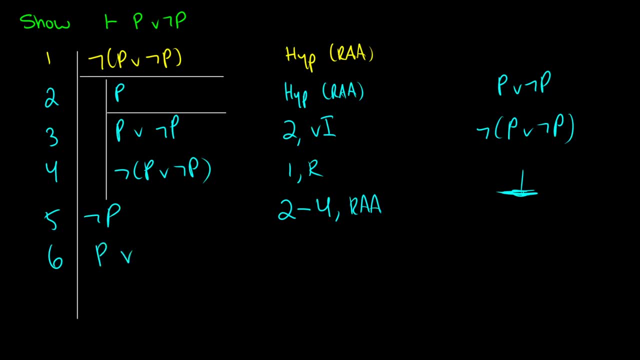 Because then in line six I can use or introduction to get p or not p. So line five or introduction: Now I have p or not p in line six and I have not p or not p in line one. So therefore in line seven I can get not, not p or not p. So this is from one to six, Proof by 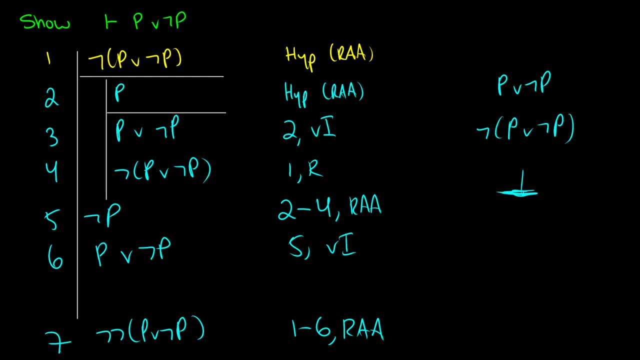 contradiction. So that's because I had not p or not p, So I can get not not p or not p. So this is from one to six, And I have p or not p here and I have p or not p here. That gives us a contradiction with those. 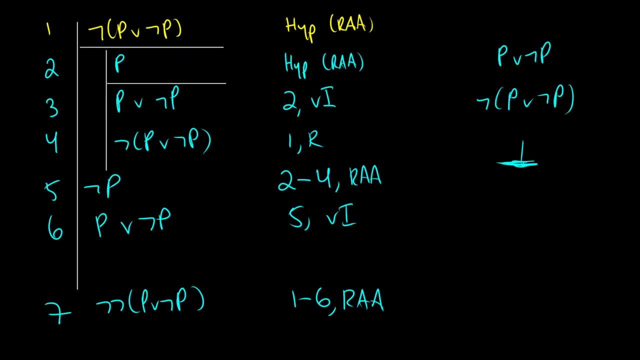 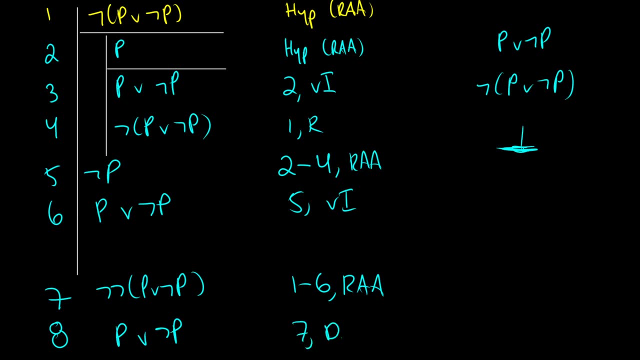 two, So we can pull those out through ra At this point. now we scroll down a little bit So that way in line eight we can use a double negation on line seven to get p or not p. So, as you can see, we're outside of the line. now we don't need any assumptions that are given to us. 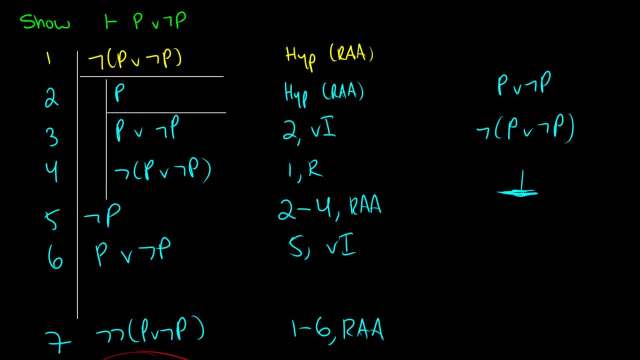 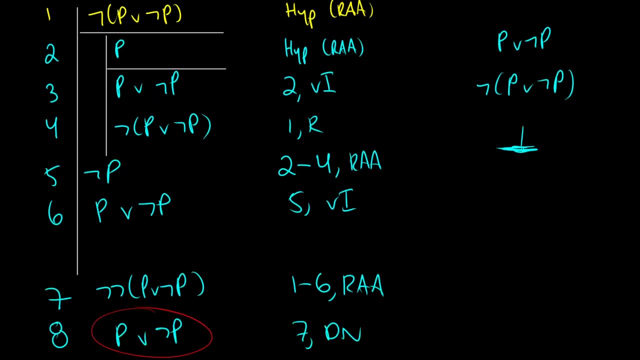 for free to do this, But we did have some assumptions for hypotheses for ra that we negated at some point and we closed off. Those are the four theorems that we can use now, at any time. Of course, there are a lot more and 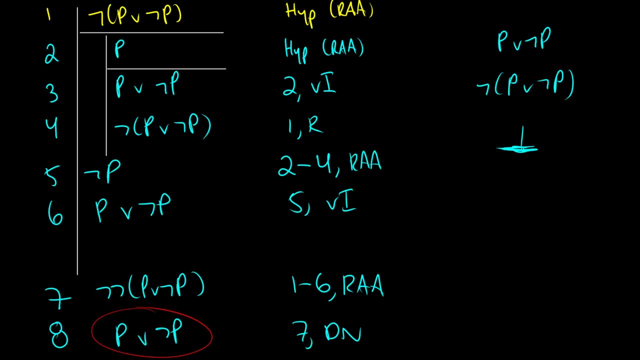 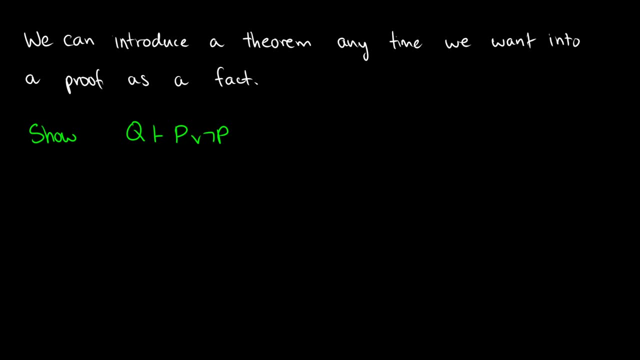 we'll do another exercise video at some point where we do some more. But the key, the important part why we do this, is that we can now introduce a theorem anytime we want to as a proof: It's a fact, It's a fact, it happens. So if we have to show, for example, that q proves p or not p,